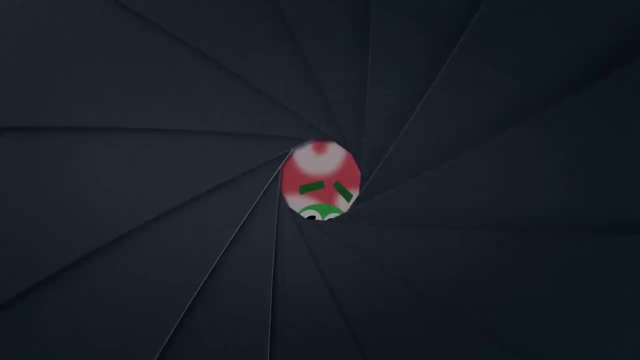 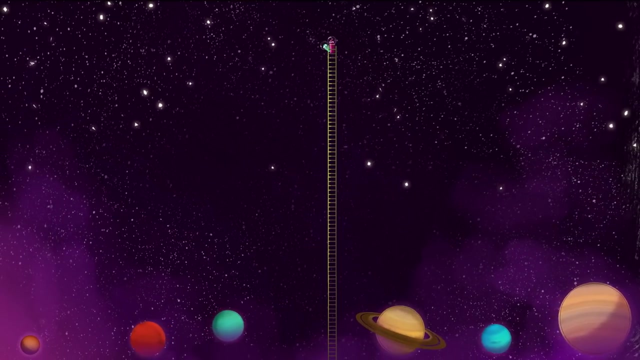 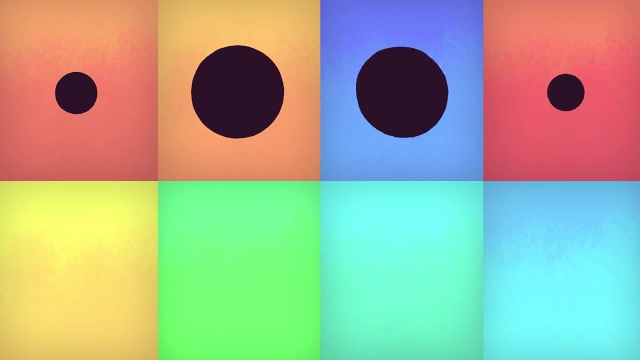 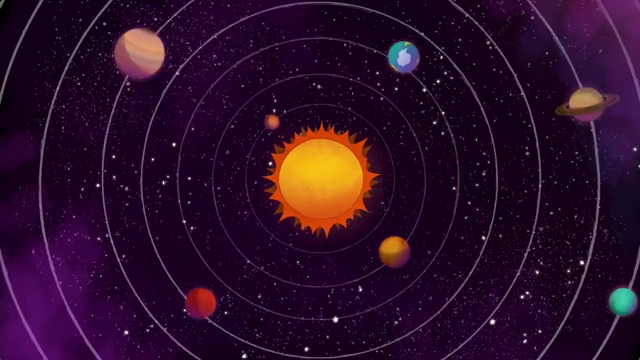 We can see the whole solar system from here. I think we can hear it from here too. We are the planets of the solar system, Different sizes for everyone. The music never ends. We are such good friends And we all orbit the sun. 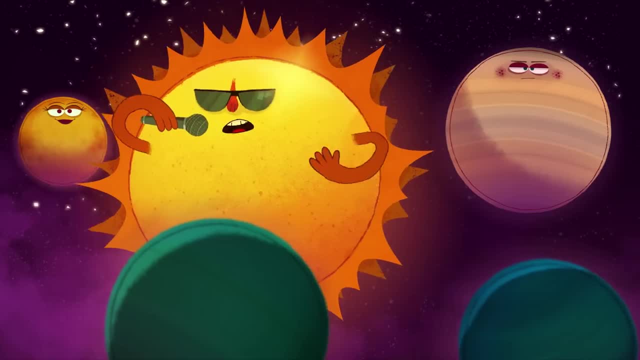 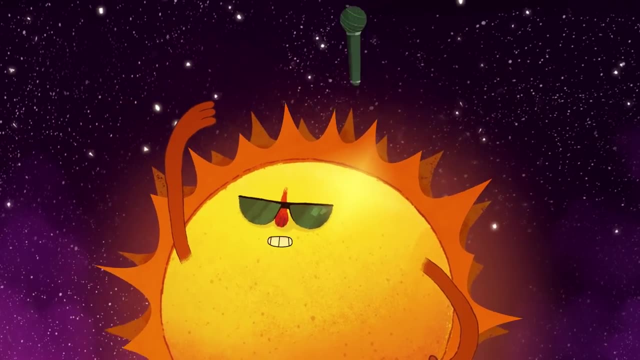 Here comes the sun rapping first on this track. from the beginning, I'm the center of the solar system. Planets be spinning around me So hot I'm roasting. you see, Now I pass a mic with the planet closest to me. 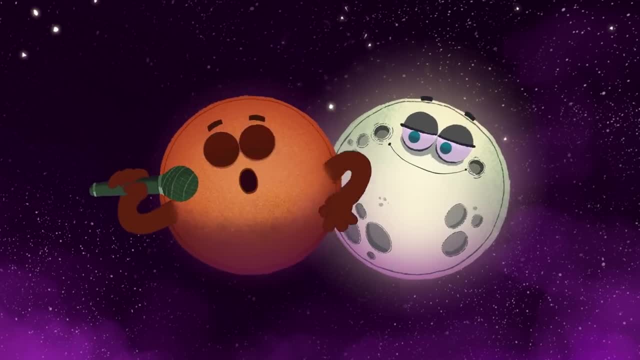 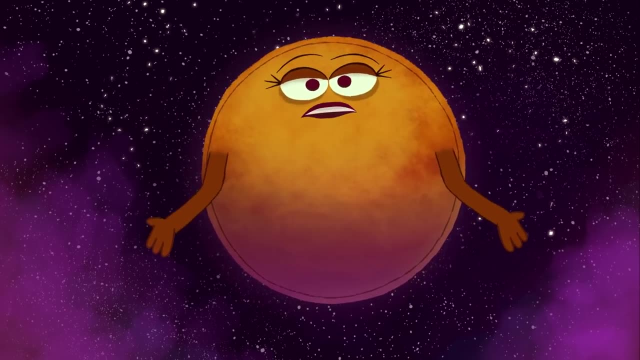 Mercury, the smallest planet, small as Earth's moon. I get super hot and cold and it's been very slow. I'm Venus. I got mountains and volcanoes that spray. I'm the same size as Earth, but spin the opposite way. 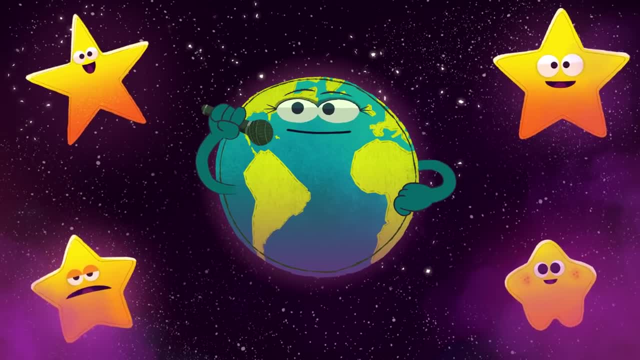 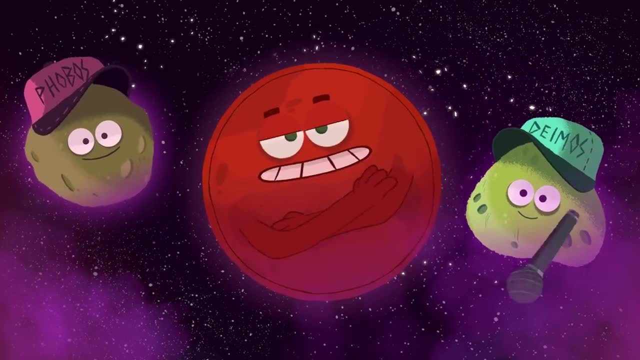 Yeah, I'm Earth. I'm the home to every boy and girl, Such a beautiful, beautiful world. I'm Mars, the red planet. I got desert tonight And I've got two moon nights. That's like one moon but twice. 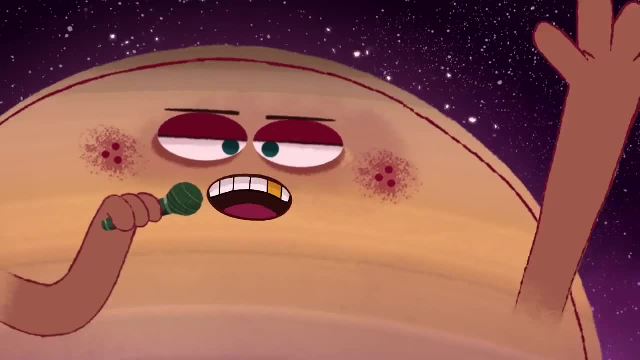 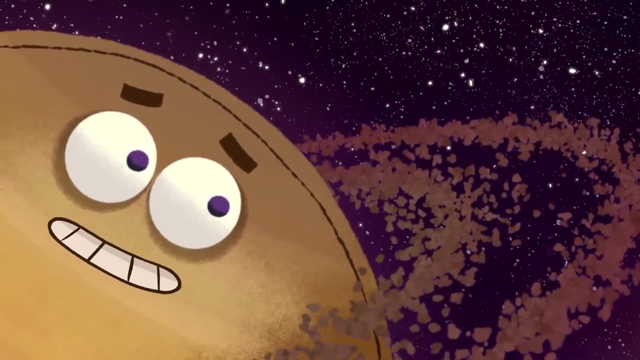 I'm Jupiter, the biggest planet. I'm humongous gargantuan. I spin the fastest, rap the fastest. Plus, I'm handsome, Blam son, Oh, please. I'm Saturn. Check out my beautiful rings Made up of billions of rocks, dust and other things. 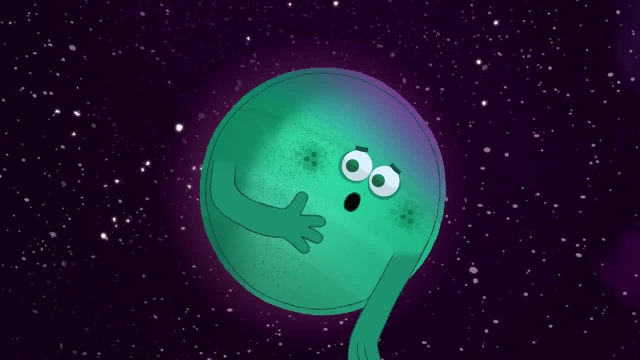 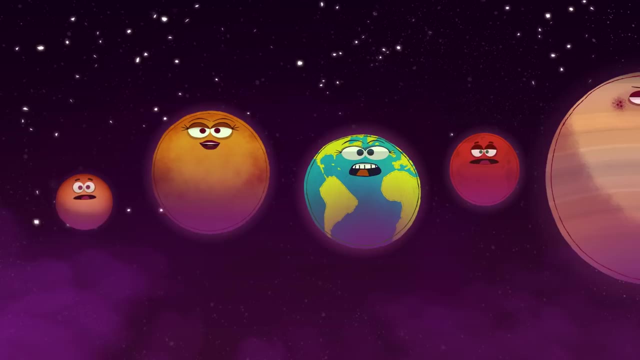 I'm Uranus. I say that with pride. Okay, I lied, I'm embarrassed because I'm the only planet lying on its side. I'm Neptune. I'm cold, dark, windy and mysterious. I'm very stormy, so bring an umbrella. I'm serious. 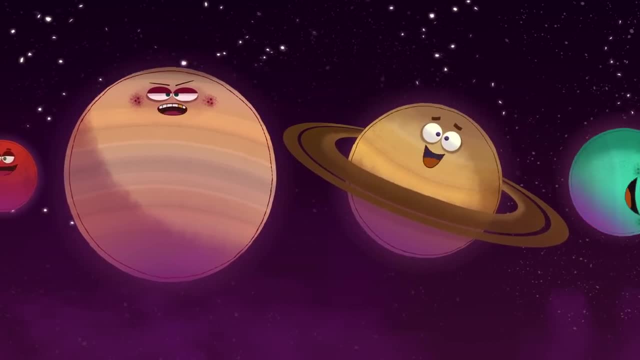 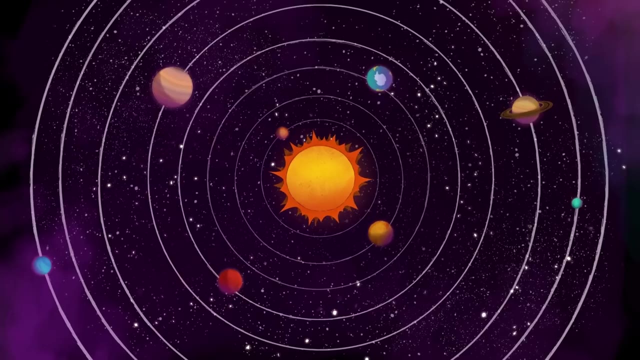 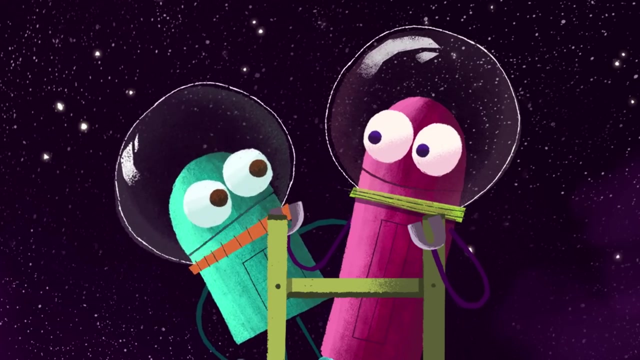 We are the planets of the solar system, Different sizes for everyone. The music never ends. We are such good friends And we all orbit the sun. Well, we are done exploring the solar system. I am thirsty. Let's explore the rest of the Milky Way galaxy. 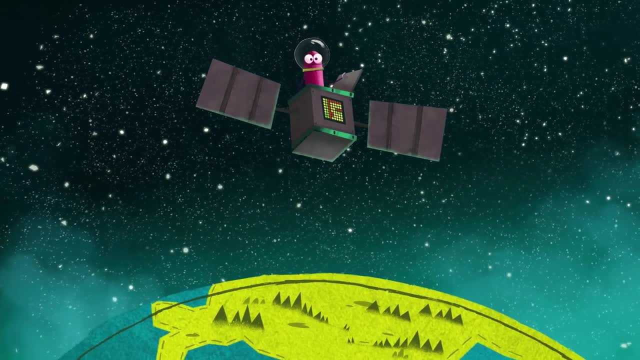 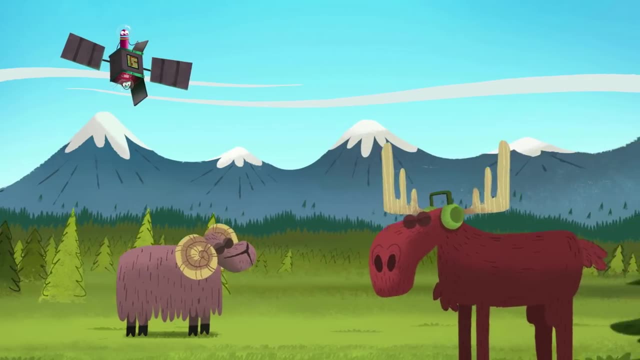 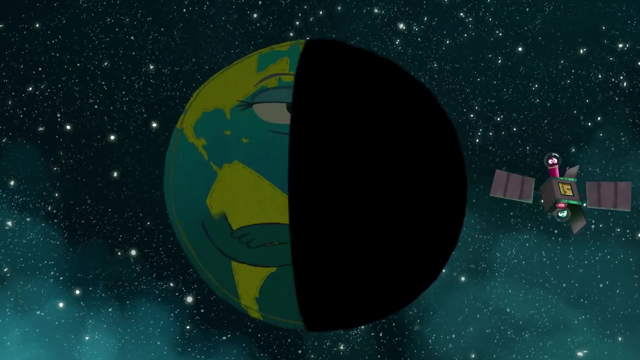 We are currently orbiting planet Earth. I'm picking up some noises, Sounds like cool music. Such a beautiful world, Such a beautiful, such a beautiful, beautiful world. I'm the Earth and for what it's worth. 25,000 miles is my dearth. 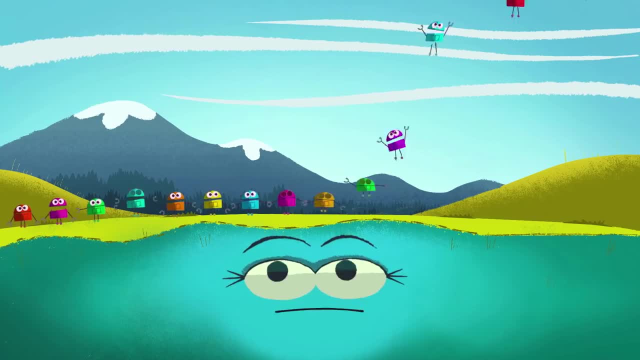 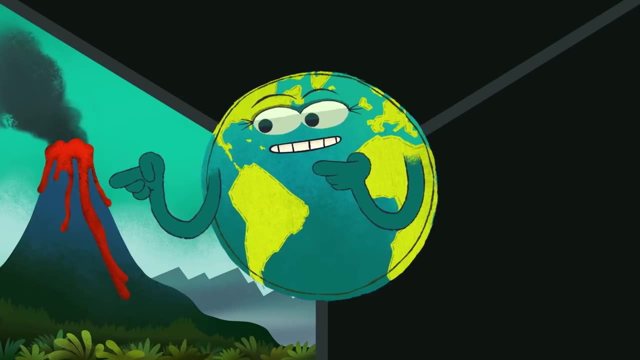 I've got more than 7 billion people living on me all across my amazing geography. Check out my mountains, valleys, trees so tall, and I got lakes, rivers and waterfalls, Volcanoes, craters, swamps with alligators, tropical islands at my equator. 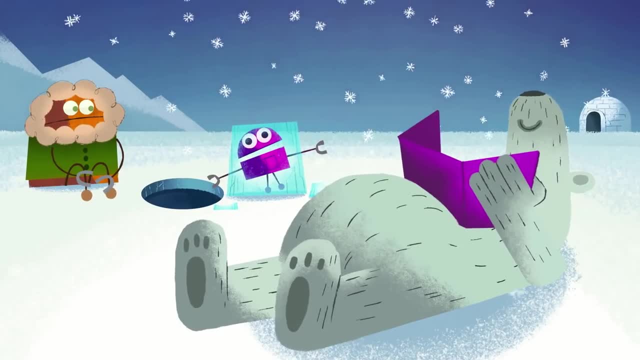 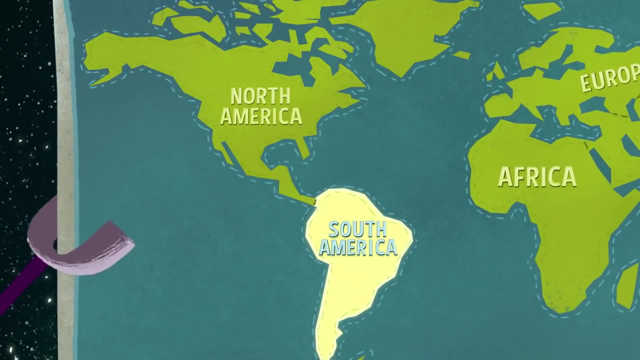 The North and South Poles. I don't have lots of ice. only polar bears say: This weather's nice, I've got so much land. yeah, I'm so immense. I've got seven. seven different continents: North and South America, Europe, Asia, Africa, Antarctica and Australia. 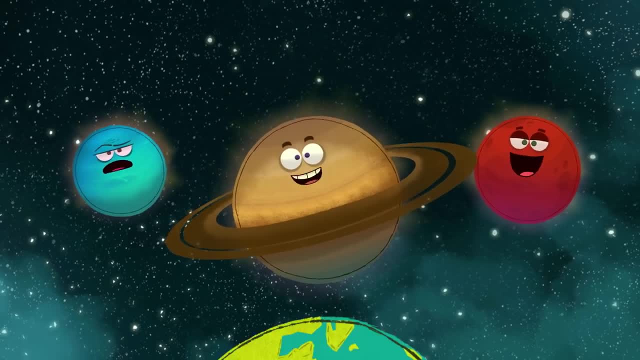 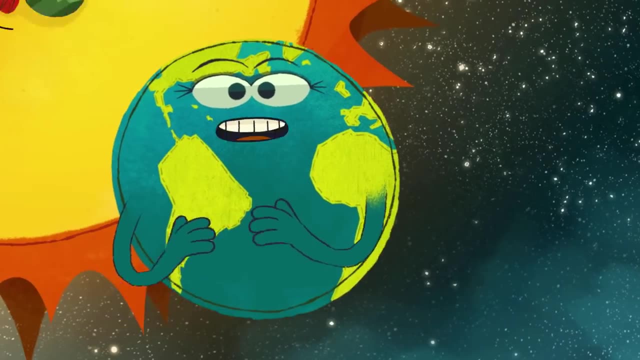 But the biggest thing everybody can see is that I've got a lot of water all over me. I have oceans with lobsters, whales, otters. three-quarters of me is covered in water. I orbit the sun. I'm so hot. 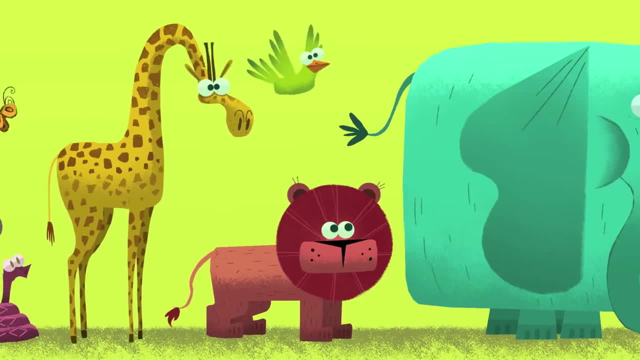 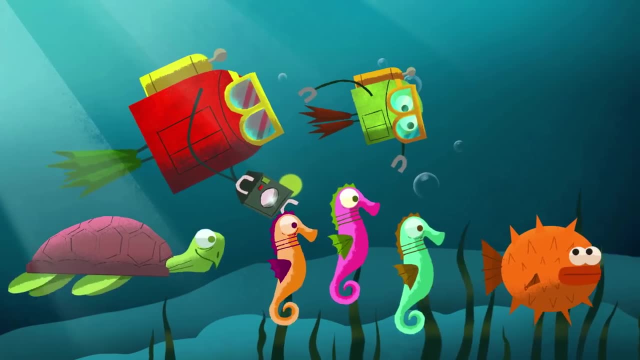 That's his line, and the moon orbits me. It's my time to shine. I'm filled with life, both big and small. I'm so hot, Both big and small. The most beautiful planet of all, Such a beautiful, such a beautiful, such a beautiful, beautiful world. 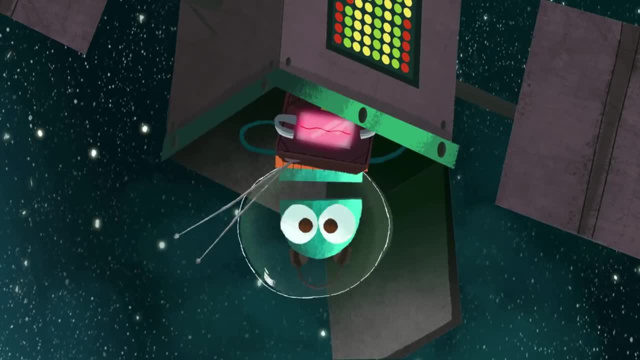 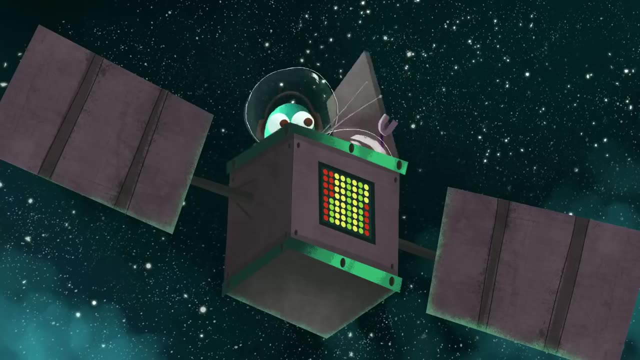 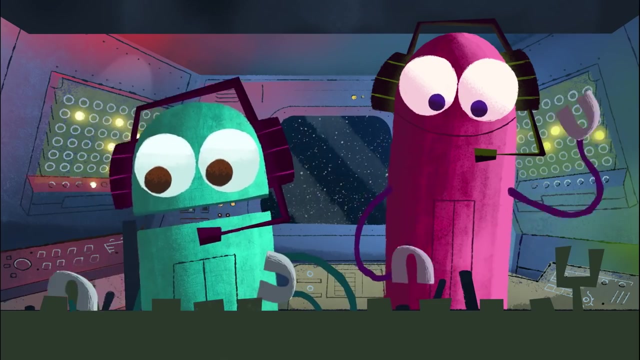 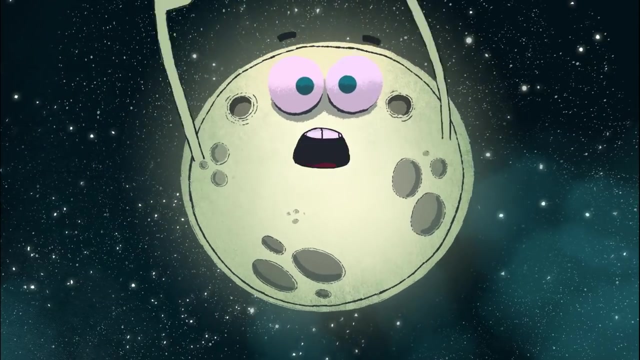 It is the home to every boy and girl. It's a beautiful, beautiful world. I'm getting homesick, Me too. Computer, take us home. We're preparing to land our spacecraft on the moon. Houston, we have a song. 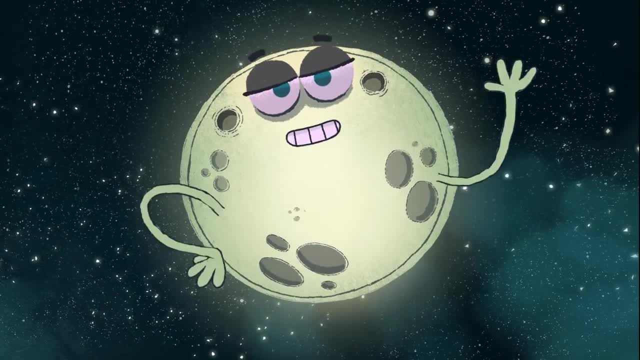 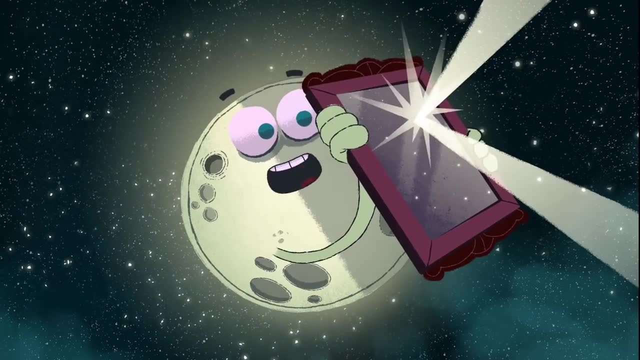 It's my time to shine. It's my time to shine. The day is over now, So it's my time to shine. Good evening, it's the moon Here to regale you with a tune. I'm so bright up in the sky at night, but the truth is I'm just reflecting light. 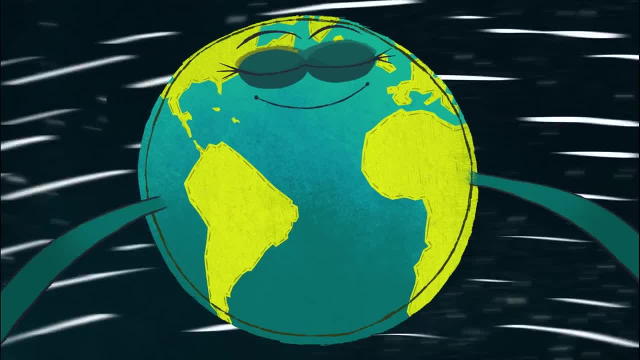 See, let me help you break it down. The Earth and I are spinning around And I orbit the moon. It's my time to shine Here to regale you with a tune. I'm so bright up in the sky at night, but the truth is I'm just reflecting light. 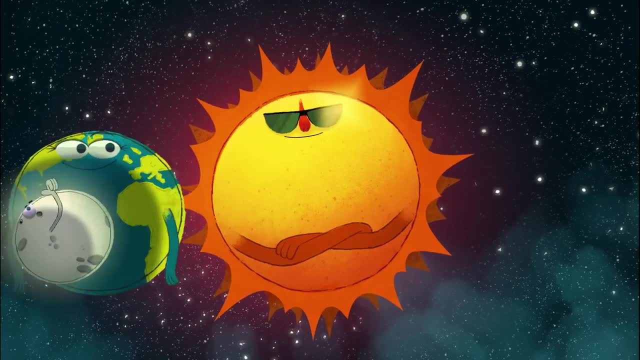 See, let me help you break it down, And I orbit the Earth in a loop. You see, the moon is kind of like my hula hoop. We both orbit the sun. He's the big shot. I'm the center of the solar system. 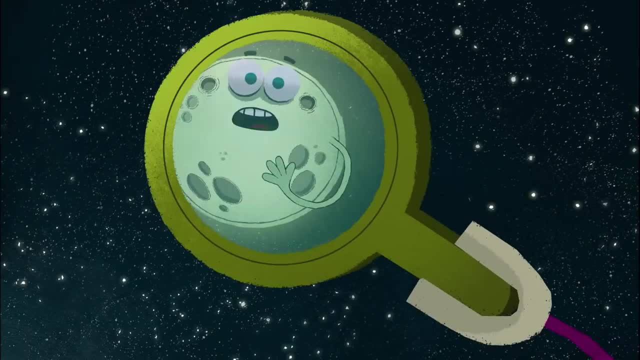 I'm so hot. The sun's like a light bulb And I'm like a mirror. Light bounces off me And then it appears to the Earth below for a lovely view For animals like wolves who go Sometimes. I'm full. 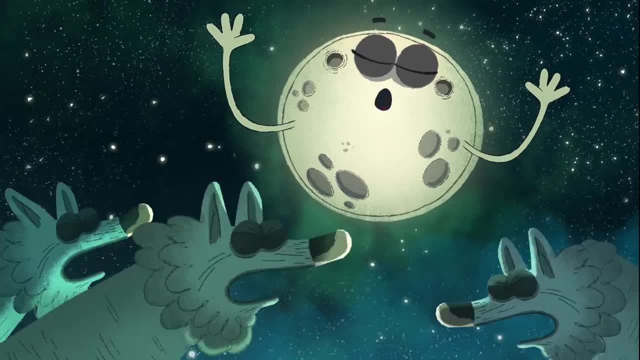 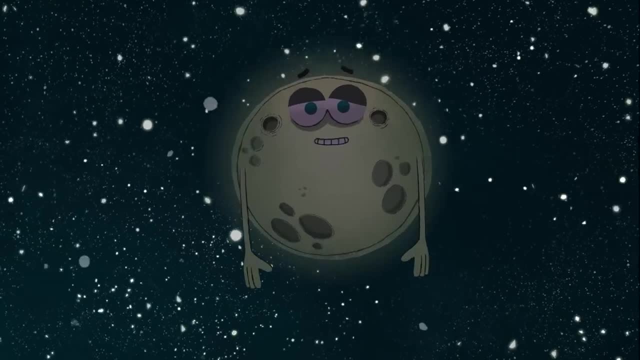 Sometimes half on, Sometimes I'm crescent Or it looks like I'm gone, But I'm here in the dark, Just a lonely moon, Hoping that somebody will visit me soon. I'm covered in dust and I'm made of rock. 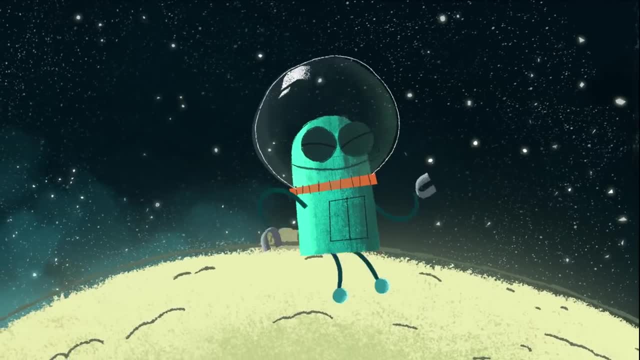 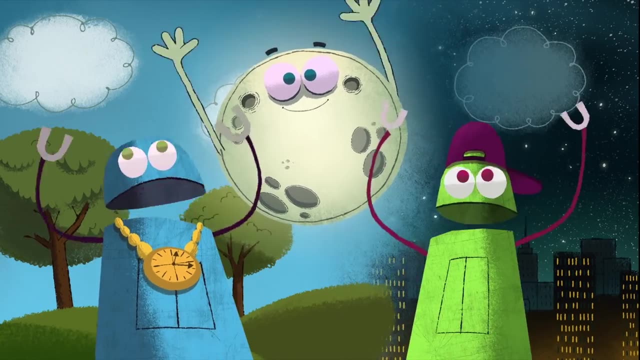 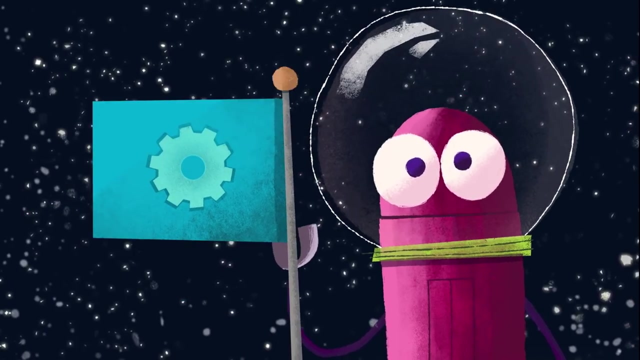 So come see me soon And go on a moonwalk. It's my time to shine. It's my time to shine. Both at night and at night we can see the moonshine. It's my time to shine. It's my time to shine. 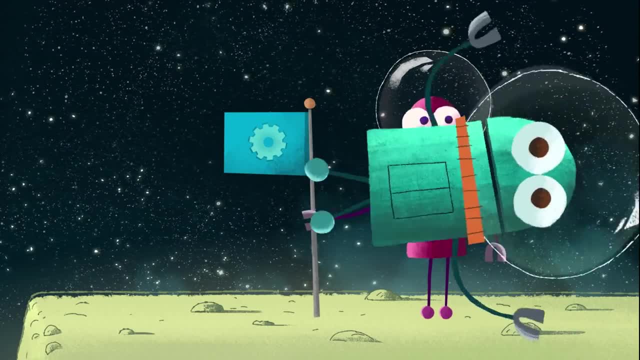 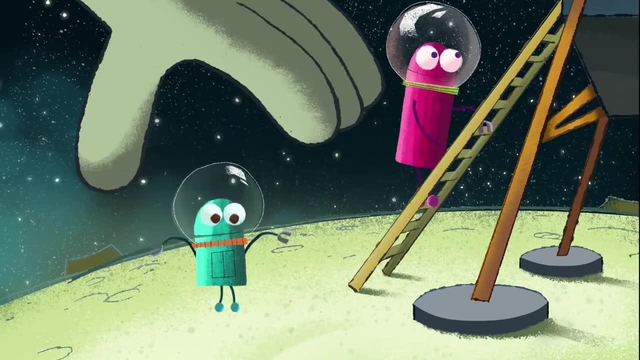 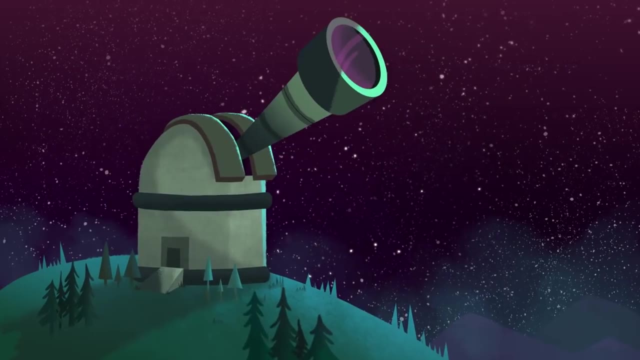 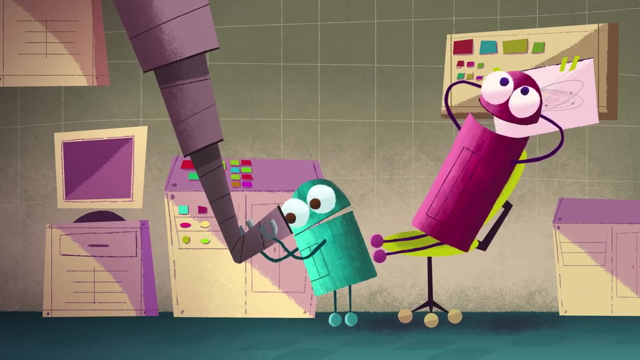 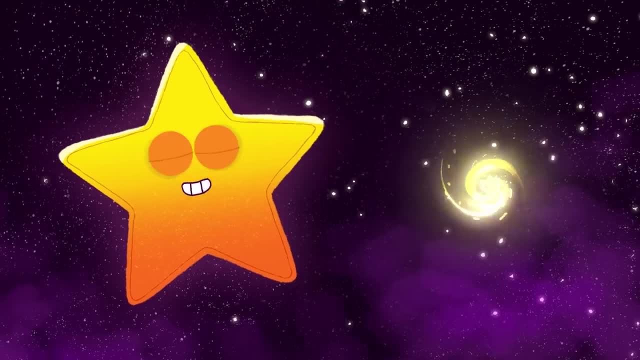 I'm a star from afar. Yes, you are, And so am I. We are balls of hot gas that shine in the sky. There are trillions and trillions of us. That's a lot. Even the sun is a star. The sun's so hot. 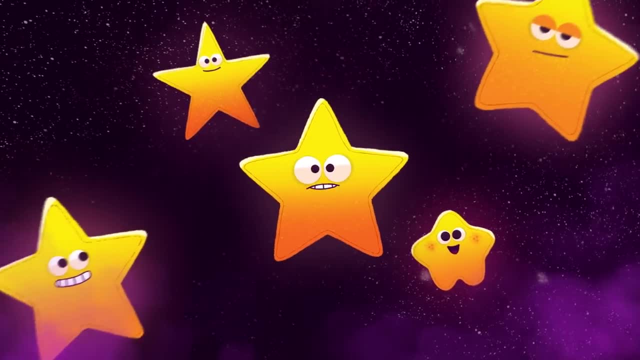 There are lots of other stars Like him And me, And me And a bunch of us together form a galaxy. There's billions of galaxies, Lots of stars, Understand There's more stars in space than all of Earth's grains of sand. 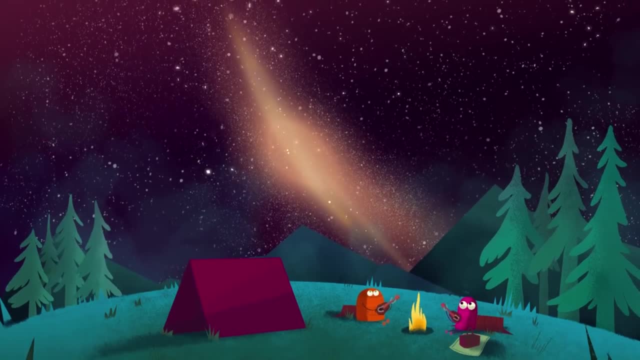 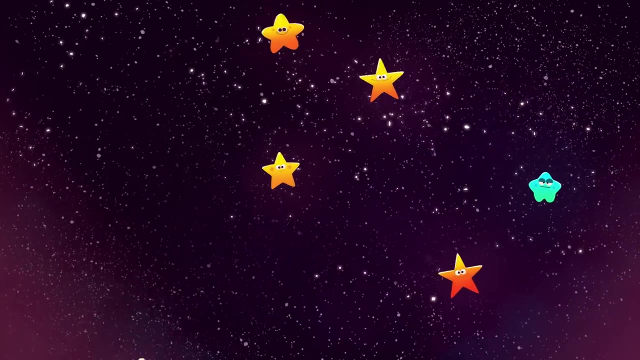 And from land, with your eye to the night sky display, You can see the Earth's galaxies, The Milky Waves, The stars are different sizes And we can morph. There are super giants, Giants And dwarfs And we form constellations Which are patterns of stars. 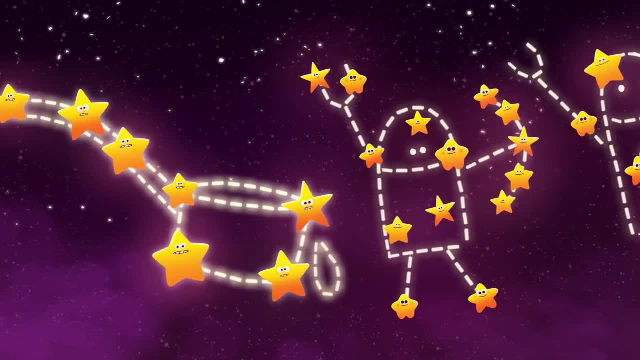 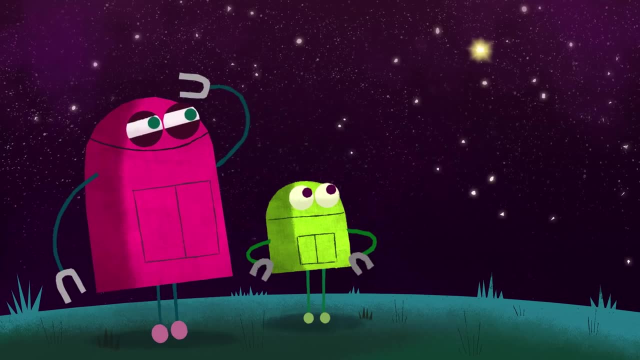 Before GPS. that's how you know where you are. We're the Big Dipper. We're the belt of Orion. We're the Gemini Twins. We're Leo the Liar. People think we twinkle, But that's not true. The light's just playing tricks when it shines on you. And shooting stars aren't stars. No, they're not. 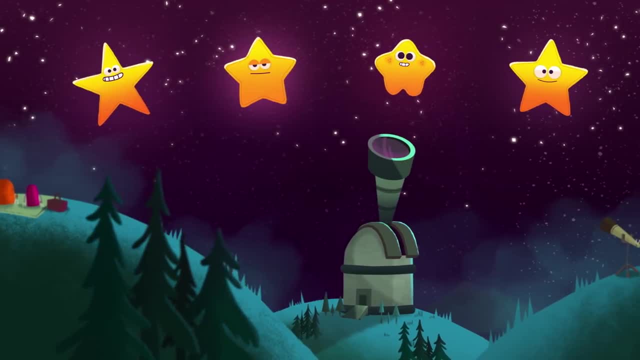 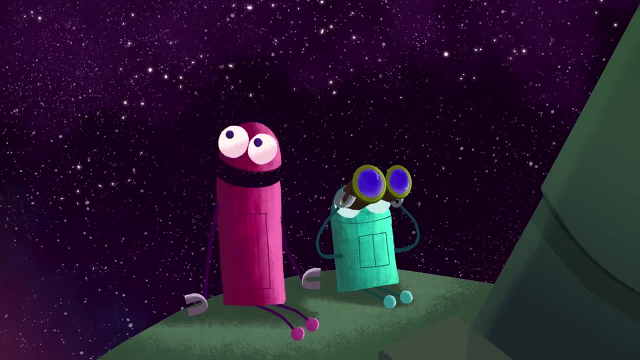 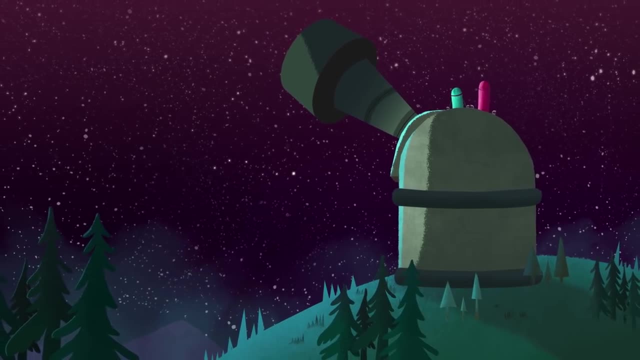 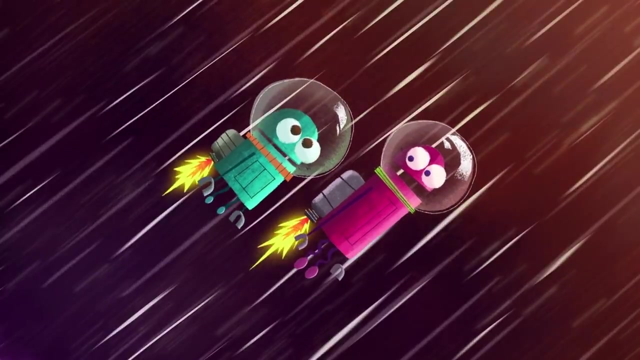 I'm a star. I'm a big, big star. There are lots and lots of stars. That's true, There really are. I made a wish. What was it? I'm not telling. According to my calculations, we are now approaching the sun. 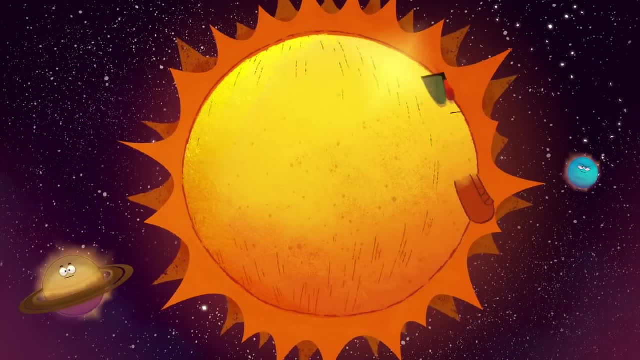 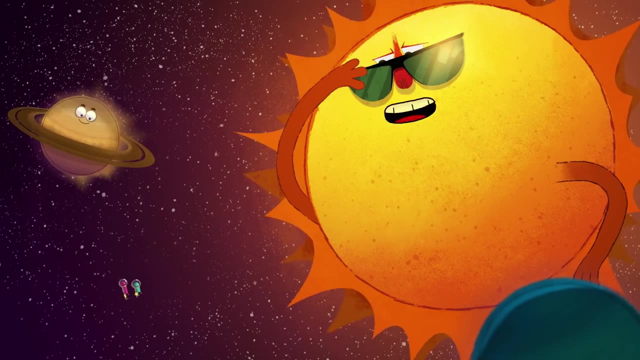 It's getting pretty hot in here. I'm so hot, I'm so hot, I'm so hot. Check me out, Check me out, I'm hot. Yo, everyone, I'm the sun. I'm made of gas like hydrogen and helium. 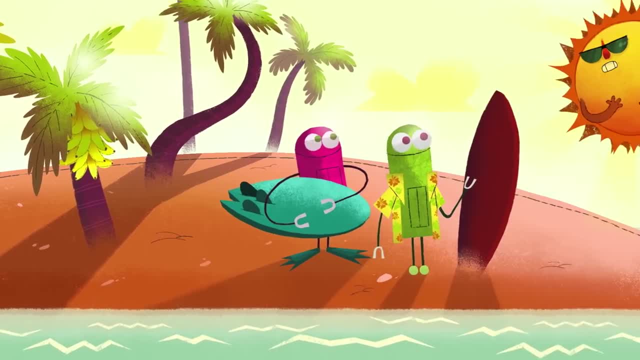 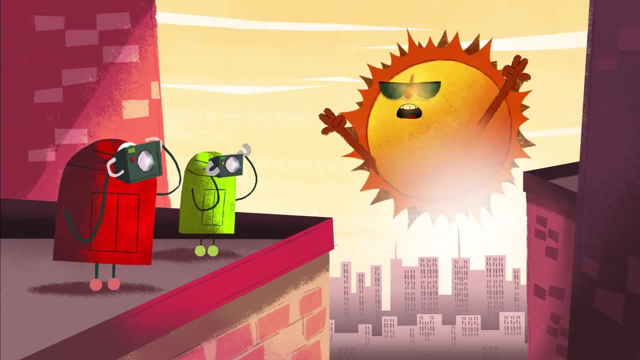 I keep the earth warm and help to grow food. I shine on the beach, on guys who say I set into the west and on comes night, And then I rise from the east with that golden light. I'm so hot, So hot and bright: 28 million degrees Fahrenheit. 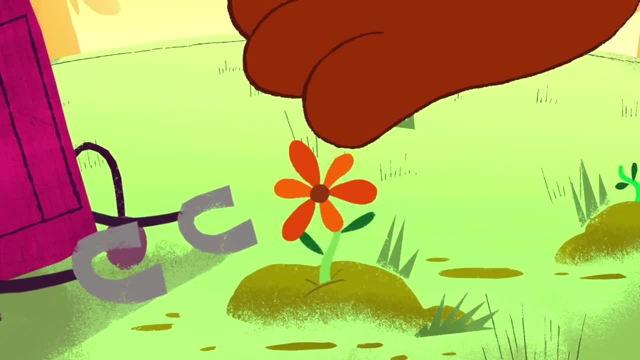 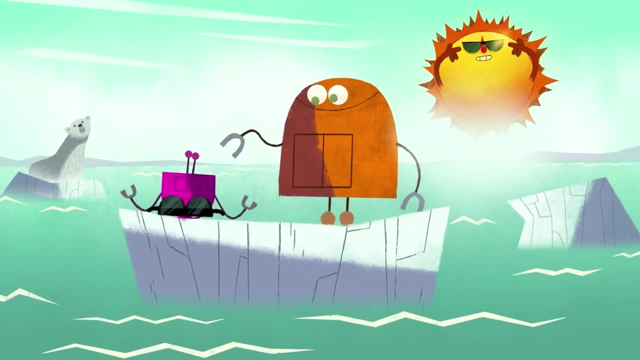 Big plants grow like trees and flowers. So powerful Got that solar power. Make the deserts dry, Make the oceans rise. Don't stare right at me. I could hurt your eyes. I'm just about a million miles wide. I'm so big you could fit a million earths inside. 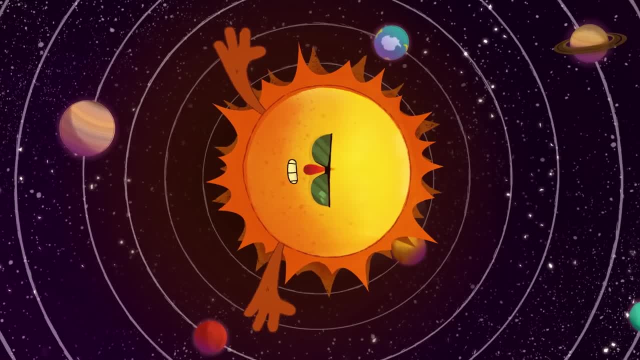 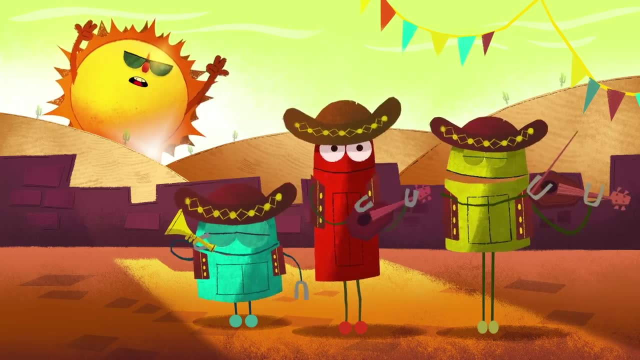 I'm the center of the solar system, Can't you see? Got so much gravity. Planets orbit me. I'm four and a half billion years old. In Spanish everybody calls me sol. When I'm not around, you'll be feeling cold. 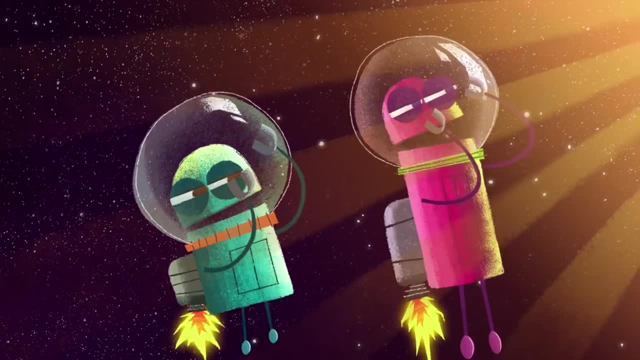 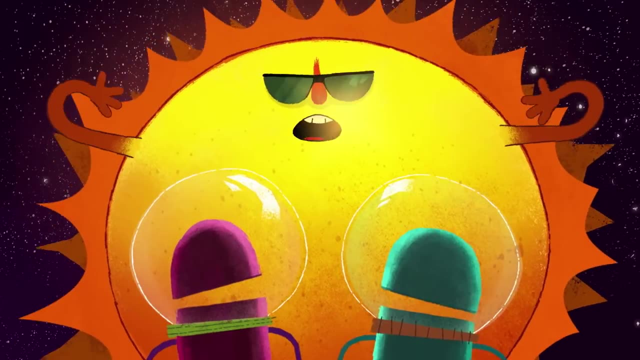 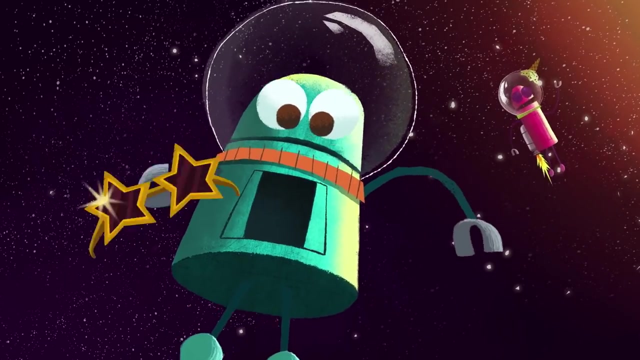 Yeah, I shine so bright with my rays of gold. I'm so hot, I'm so hot. Oh, he's right, He's really hot. Come on, storybots, Show me what you got. How hot am I So hot? The sun is so hot. I have to wear these Now. I'm cool, So cool. 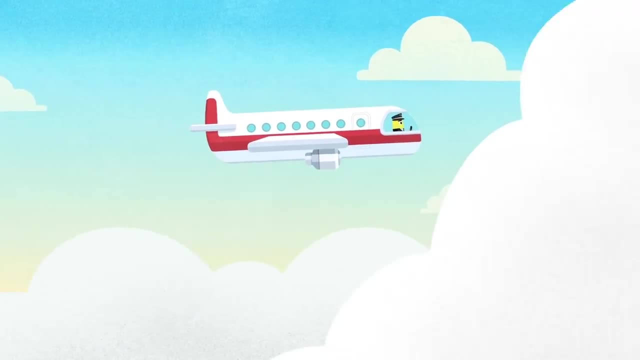 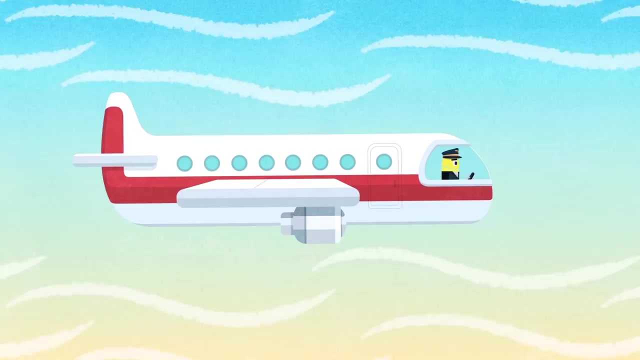 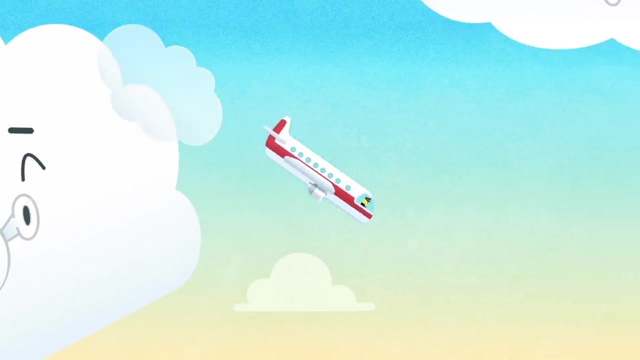 When people are taking a trip on a plane, they need someone there at the wheel. A pilot has the training and the skills to fly so that everyone is safe when they go up in the sky. The pilot keeps watch on the speed and the fuel and looks out for wind and for rain. 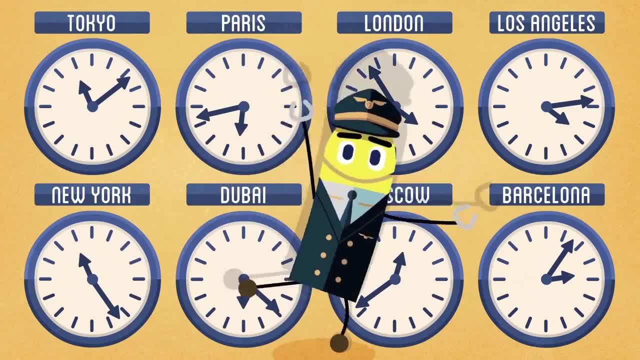 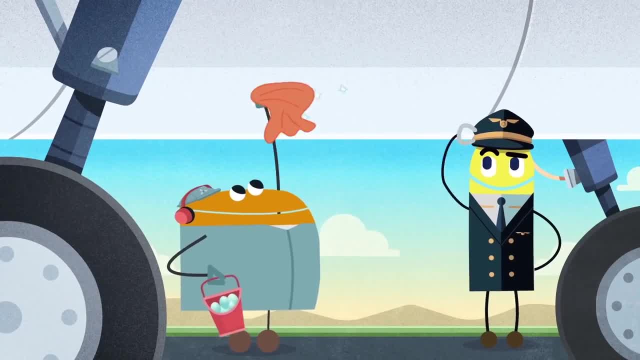 In daytime or nighttime. whenever it's flight time, the trusty pilot flies the plane. Now, before every takeoff, the pilot must check to be certain that everything's fine. The wings and the engines have to work just right from the moment of the takeoff to the end of the flight. 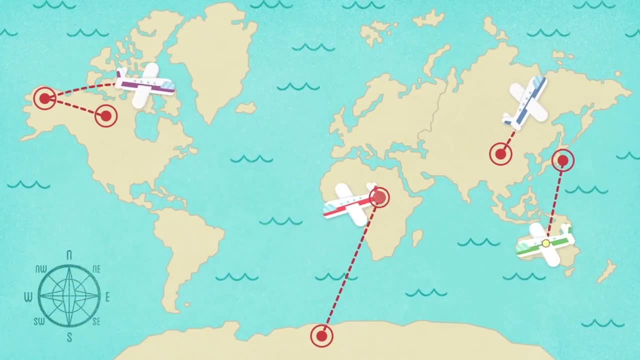 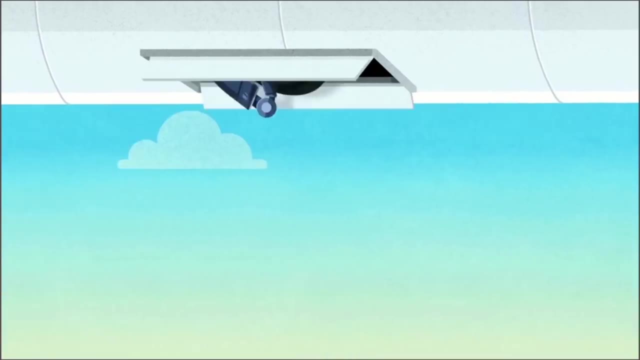 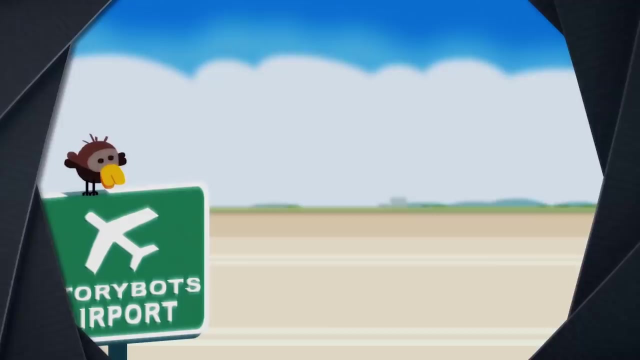 The pilot makes sure that the plane's on its course to New York or Chicago or Spain. When your job keeps you soaring, it never gets boring. The trusty pilot flies the plane. Yes, the trusty pilot flies the plane. Here we go, Hooray. 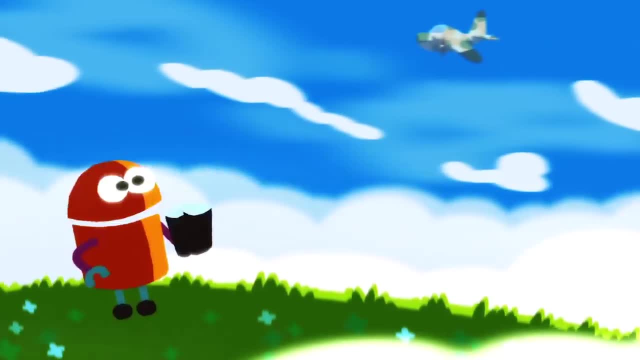 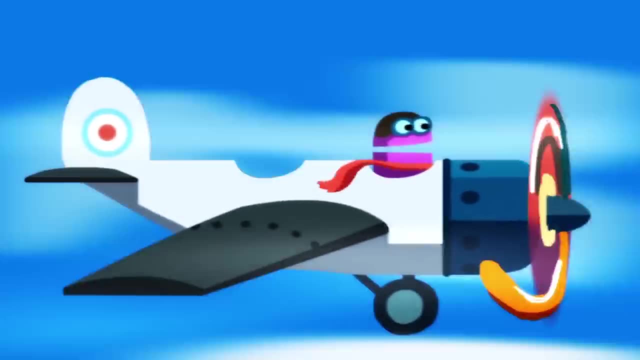 Airplane, airplane, airplane, Airplane, airplane, airplane- Up in the sky, Up in the sky, We can fly if we try. So high in an airplane. Oh my, So far, far, far up above the trees. 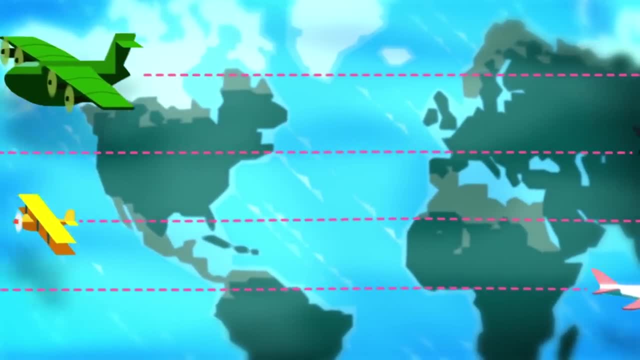 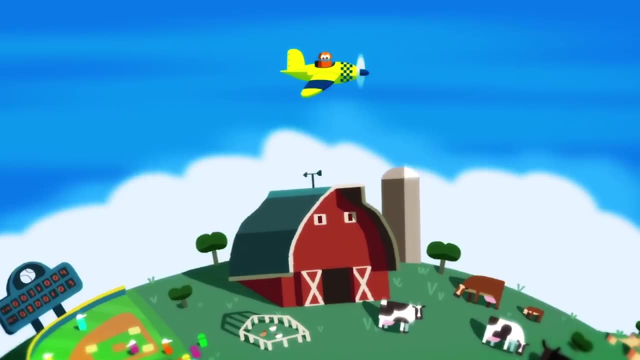 Up above the trees, We can cross oceans and seas If you please in an airplane. Yes, please, Looking down on roads and towns, Baseball fields, barnyards and cows Canyons, castles, camping grounds, Swimming pools, grammar schools. 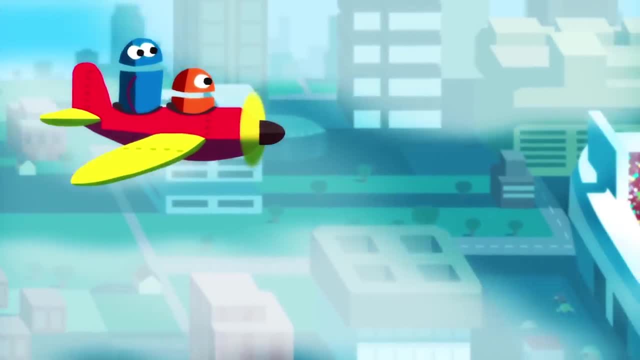 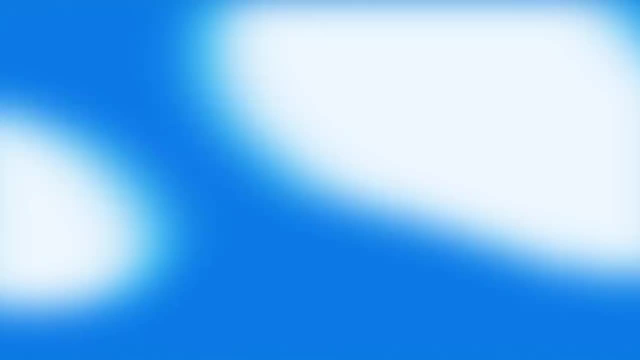 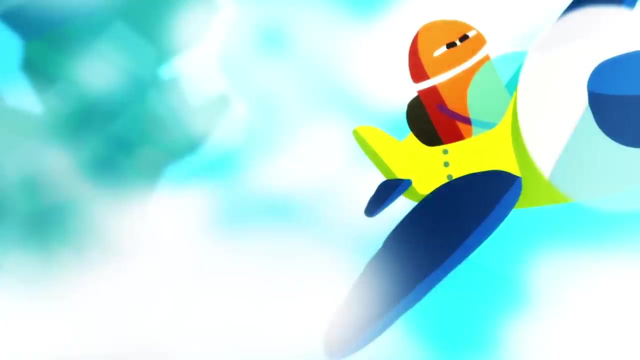 Come along to the pool. yeah, Look at all those ants. That's a football team Touchdown Airplane, airplane, airplane- Up in the sky. Up in the sky, We can fly if we try So high in an airplane. 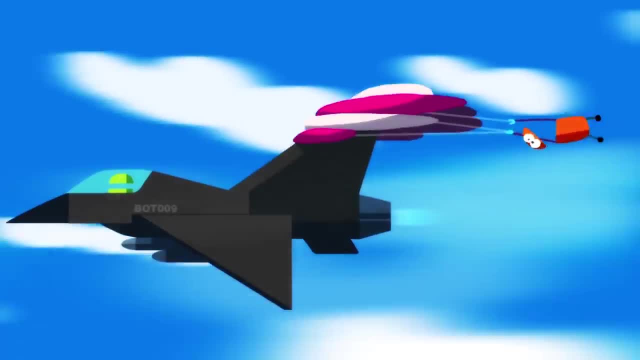 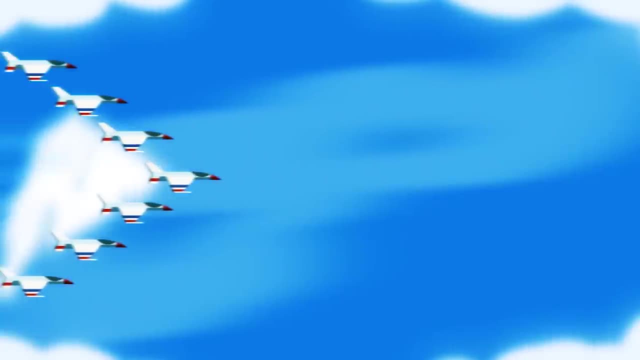 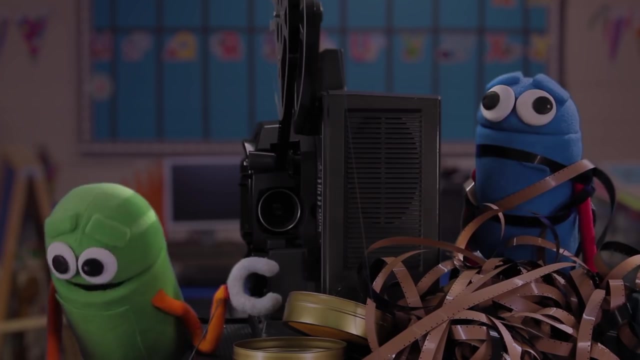 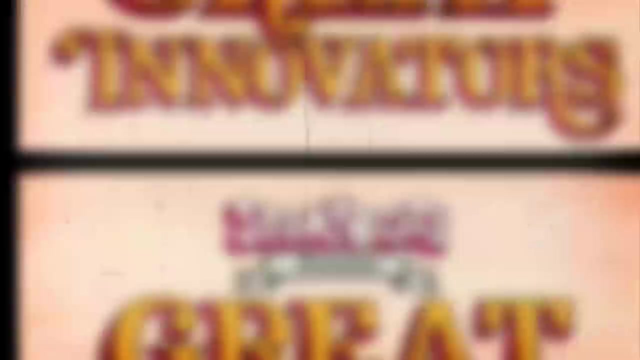 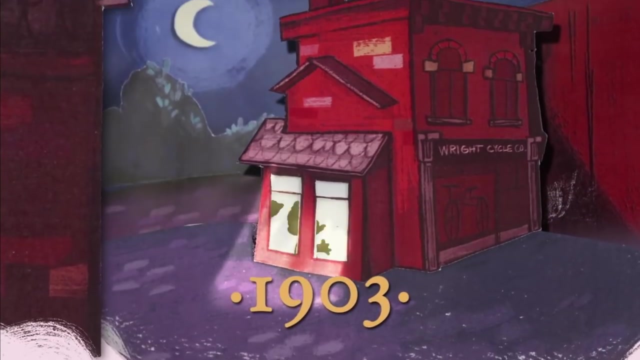 We can fly in an airplane Airplane. It's an airplane Airplane Airplane. Storybox presents Wright Innovator Wilbur and Willis, Two brothers named Wright, once dreamed of machines with the power of light In a little backroom of their bicycle shop. 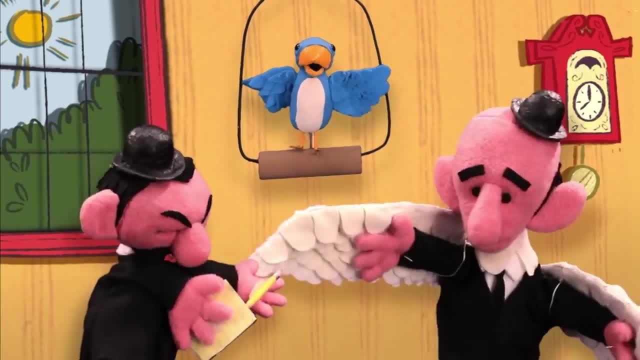 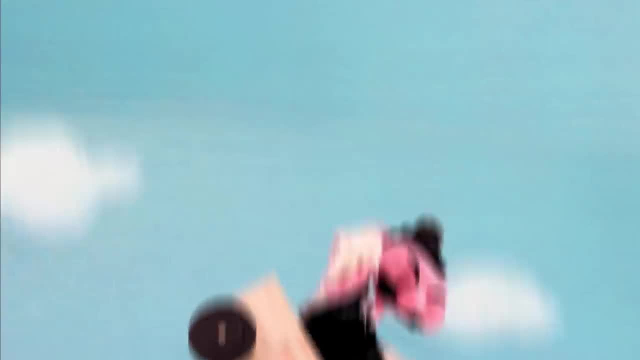 their designing and tinkering just wouldn't stop. They'd study the wings and the motions of birds When the neighbors would laugh: What a couple of nerds. they tested one glider And then built another. We're learning, said Wilbur. 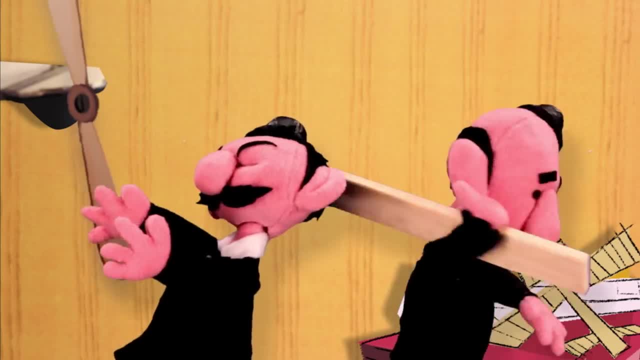 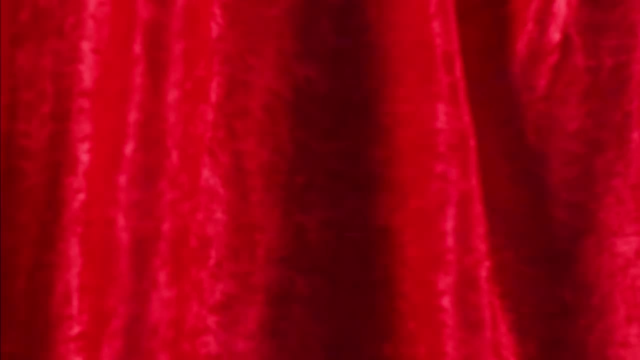 And how said his brother? They both got a bump or a bruise now and then, but they never gave up. They just tried again till at last they had built something no one had seen. They were ready to test their flying machine. 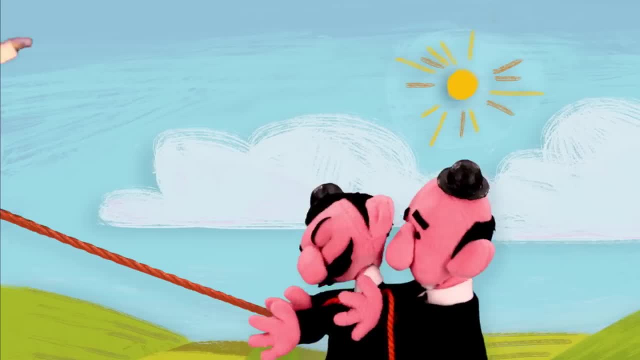 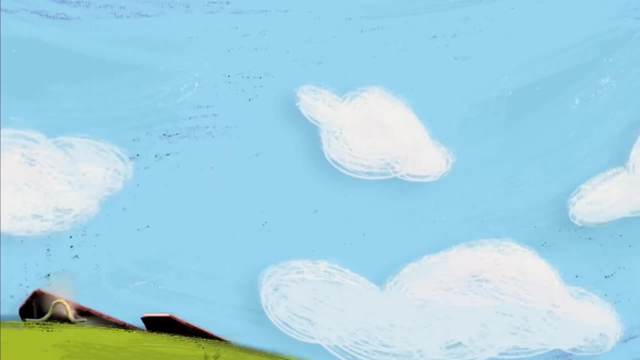 So on a day in December in 1903, near the city of Kitty Hawk, down by the sea, they cranked up the engine. And what did it do? It sputtered, It rumbled, Then zoom off, it flew. 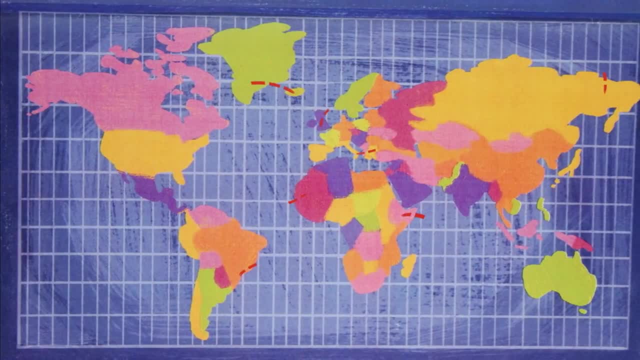 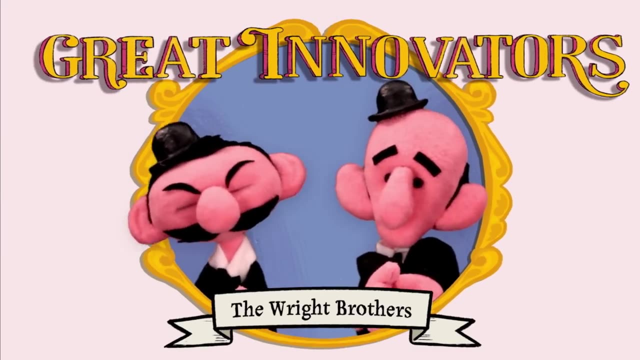 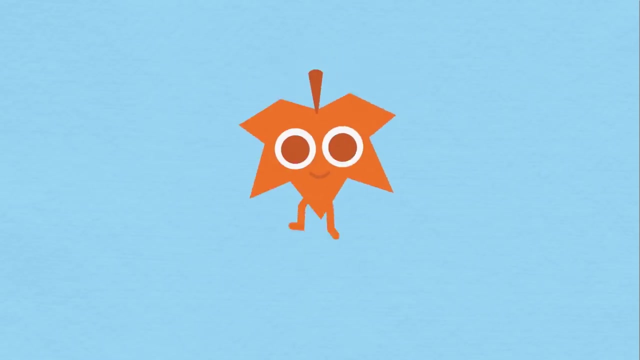 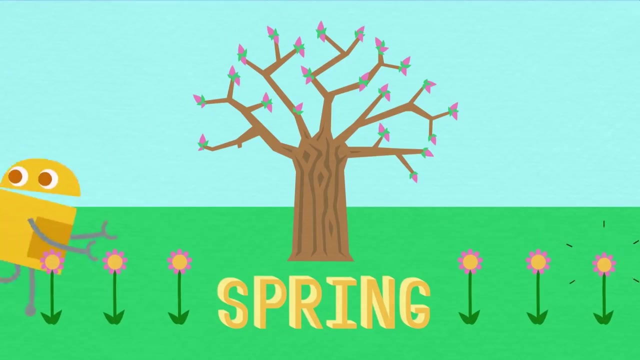 And that's why today you can hop on a plane to Chicago or Phoenix, Australia or Spain. So whenever you look at an airplane in flight, just remember the tale of two brothers named Wright. Cold weather's kind of winter's thing. In spring the plants get back their bling. 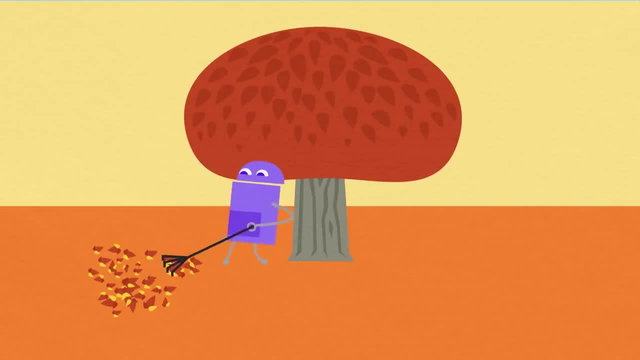 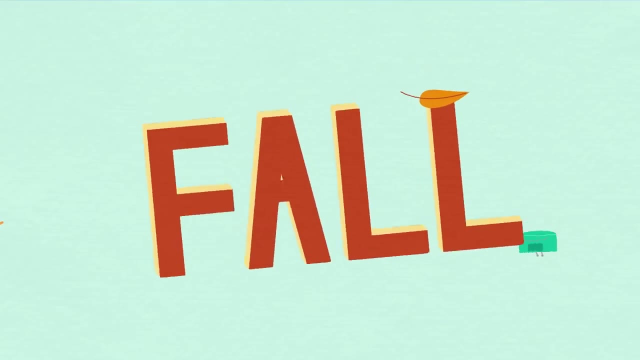 By summer they're in full swing, But in fall they're long. Leaves go tumbling down, down, down to the bottom. Oh, that reminds me Some folks call fall autumn. Well anyway, Winnerspring, summer fall. 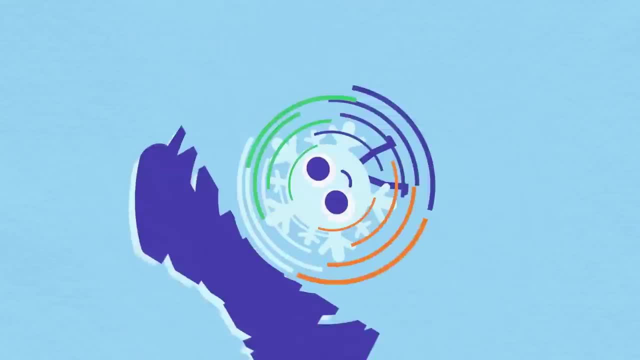 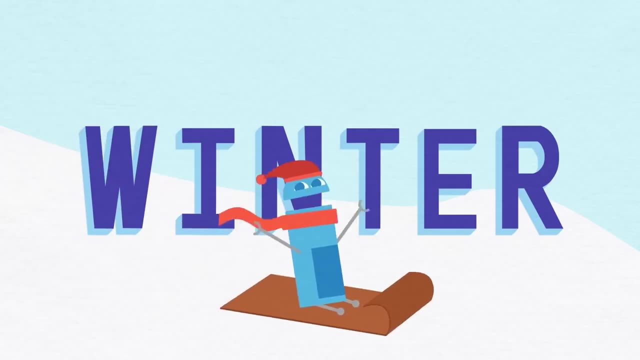 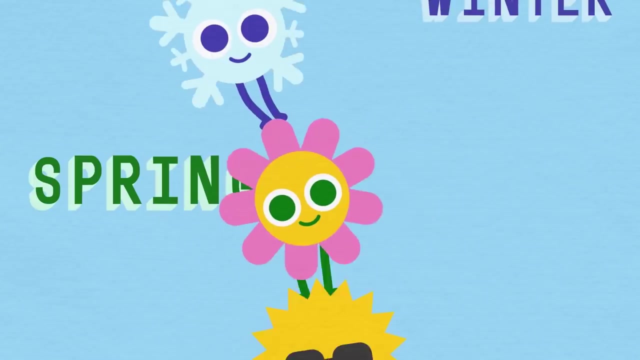 One year, four seasons in all: Winnerspring, summer, fall. Four seasons, you can count them all: Winnerspring, summer fall. One year, four seasons in all: Winnerspring, summer fall. Winnerspring summer fall. 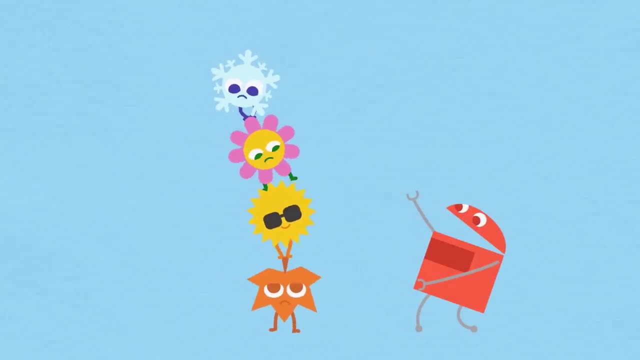 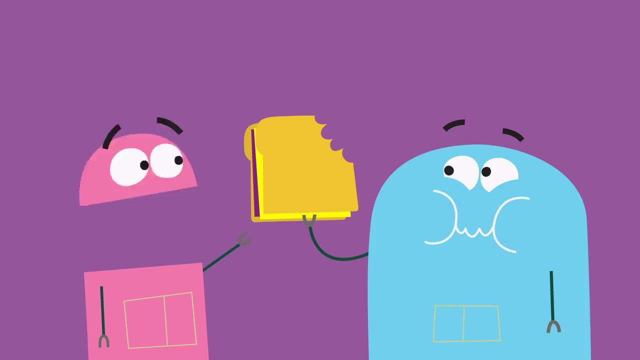 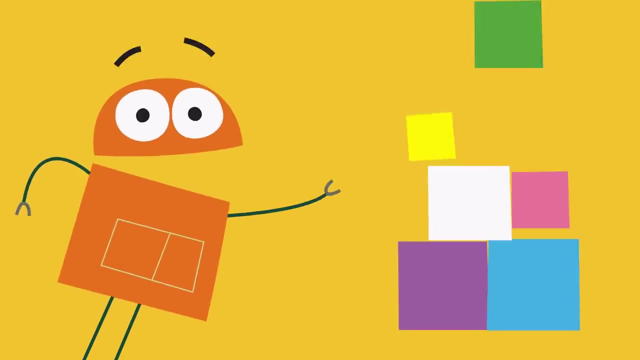 Summer, fall, and now you know them once and for all. What is that square that you are eating? It is called a peanut butter and jelly sandwich. Squares, squares, squares, squares. See them here and see them there. Squares, squares, squares, squares. 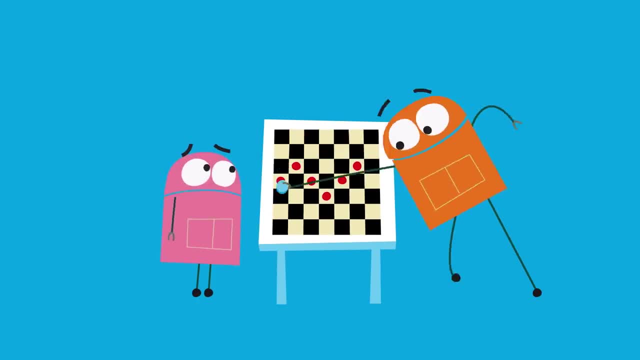 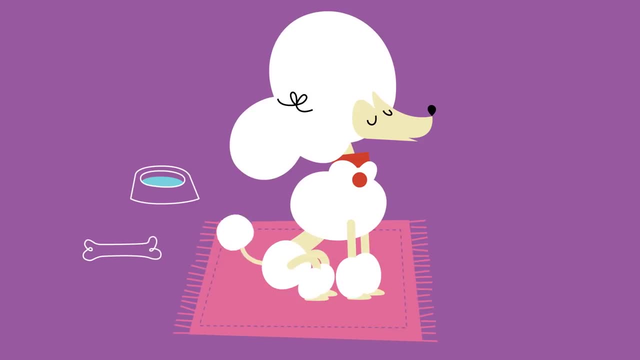 Squares are everywhere. A checkerboard is a square. A hopscotch court is made of squares. This cracker is shaped like a square. Squares are everywhere. Can you grow your poodle's hair in the shape of a square? 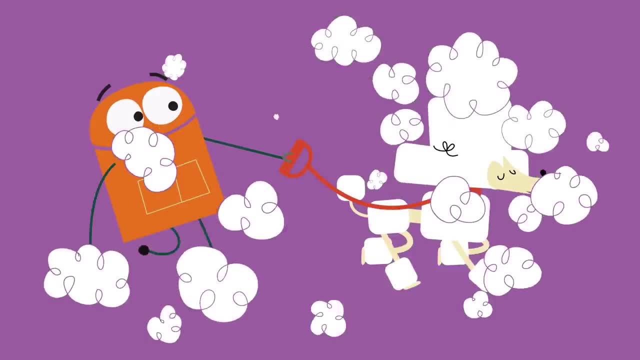 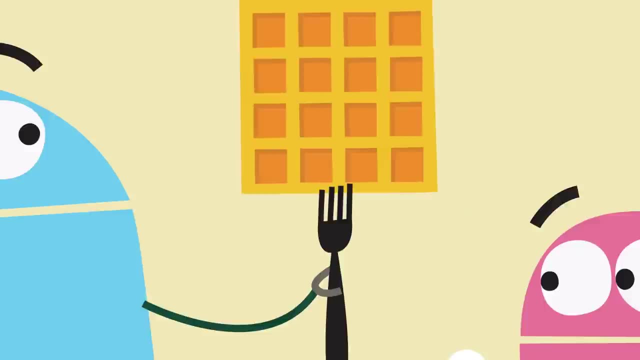 Oh, yes, you can, but you've got to take some care, And you must beware that some people might stare Lucky bear If your poodle's hair is square. My waffle is completely square And it is made up of many tiny squares. 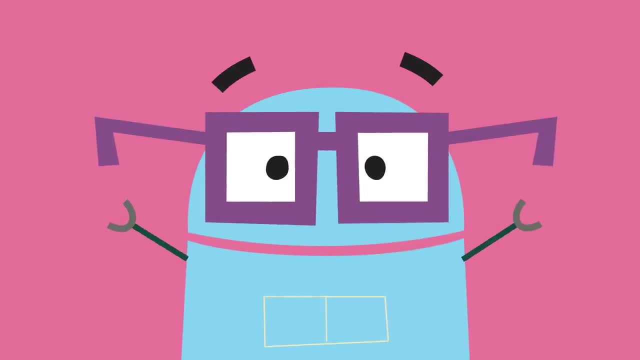 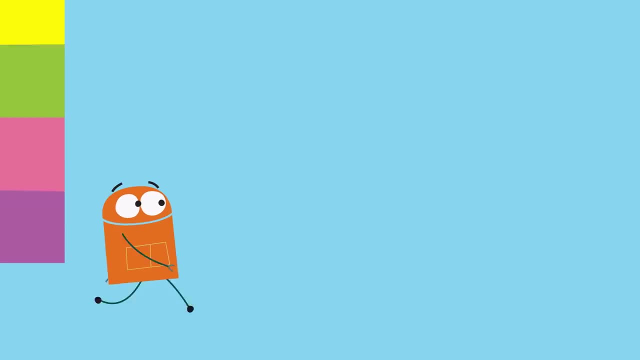 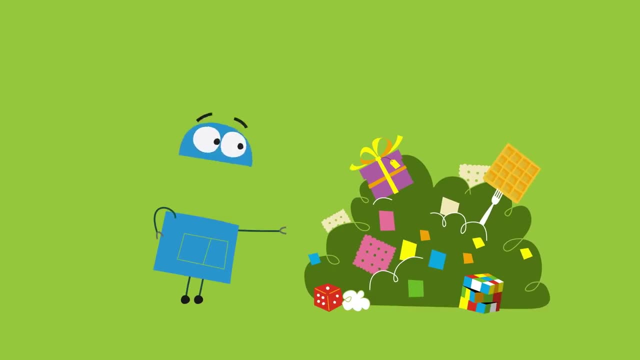 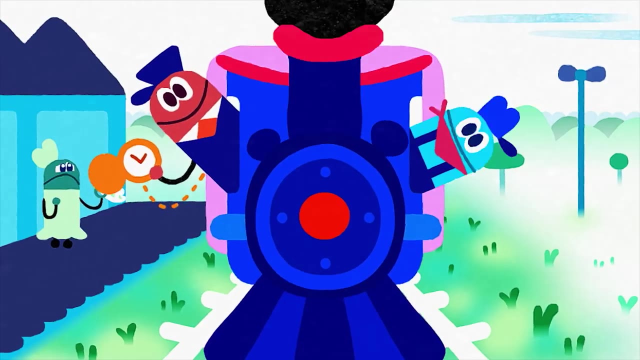 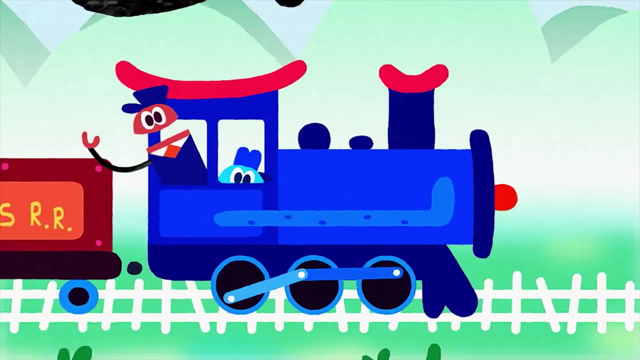 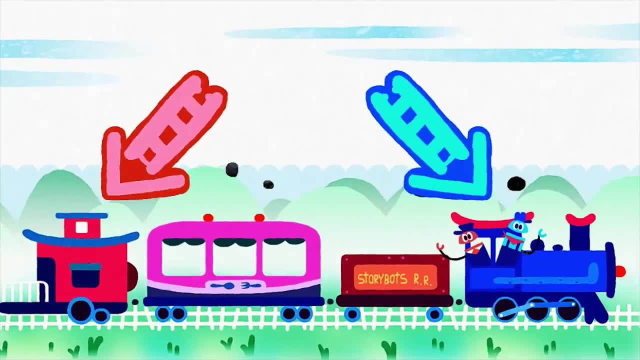 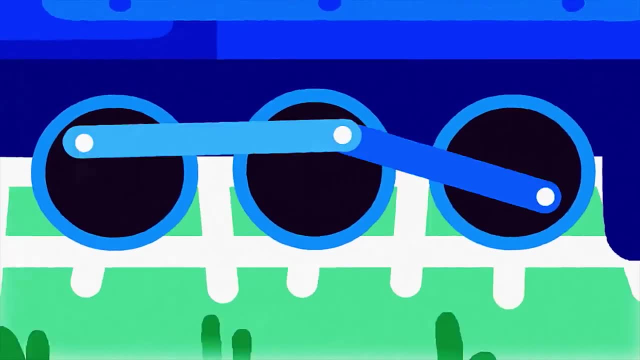 And there's the engineer. Hello, In front's the locomotive, The caboose is in the rear. Back here, Middle is the dining car for when you need a snack. I'm hungry. We're warring across the country. Just hear those wheels clack. 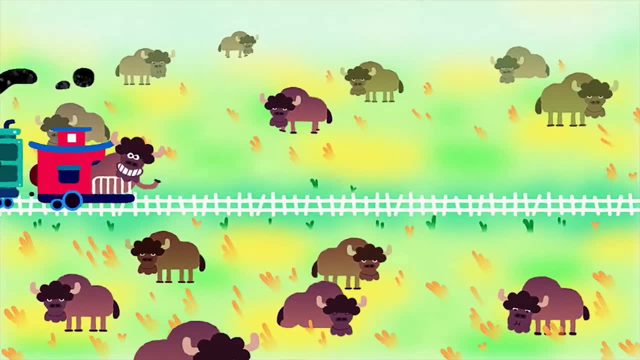 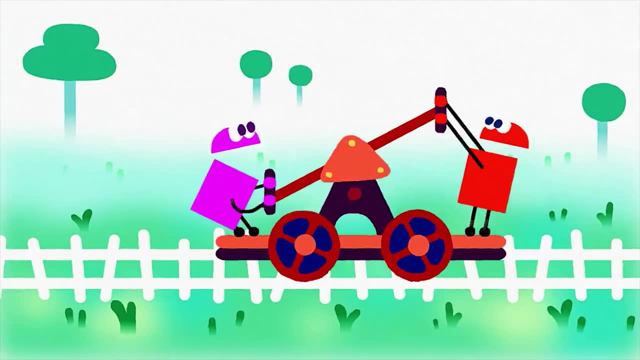 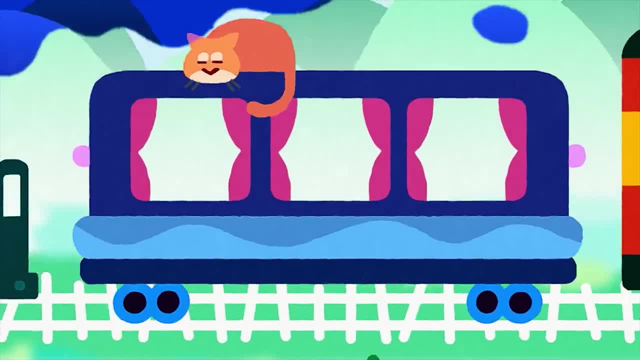 The box car's full of cans of beans. The flat car's hauling lumber. The sleeping car is for those long trips when you need to slumber. The observation car's windows are big, so you can see. The observation car's windows are big, so you can see. 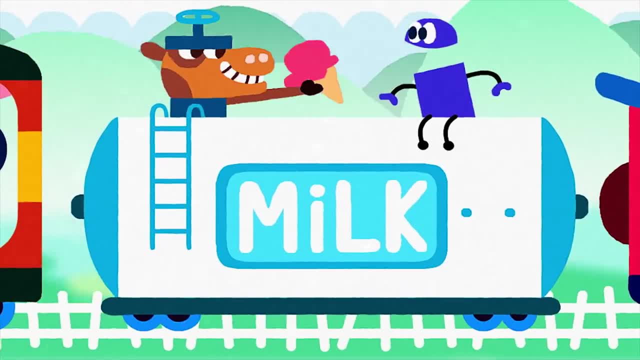 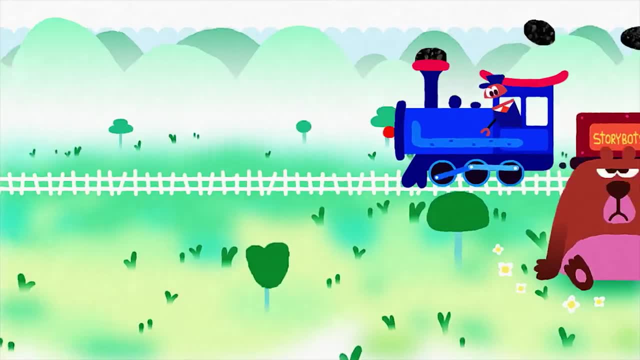 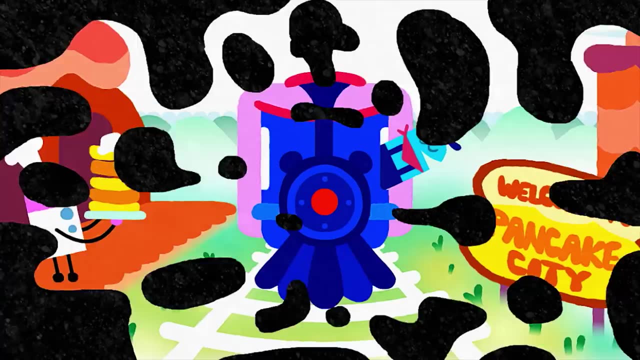 Yo train ride. lookie, there, There goes a building, there goes a bear. See a moose and a lady in a rocking chair. We're riding on a train. We're riding on a train. We're riding on a train. 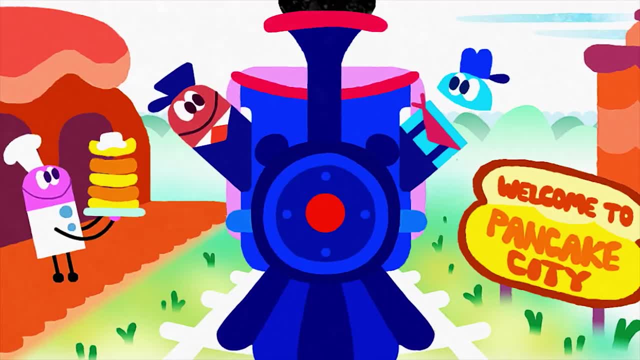 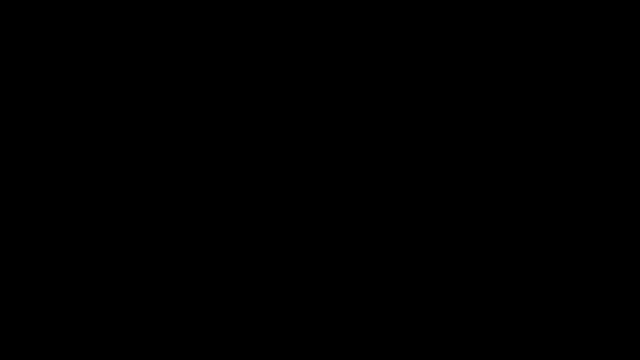 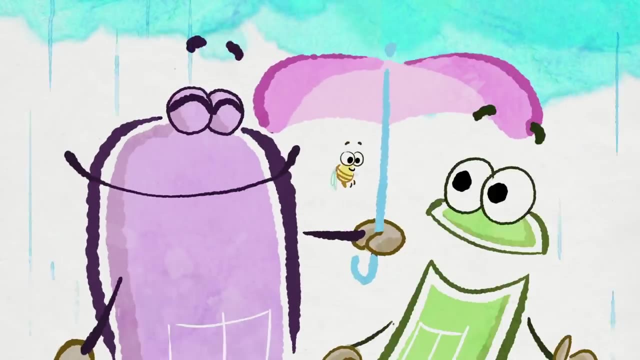 Did you see that moose? No, I fell asleep in the dining car. Sorry, Max Ta-da. Just like the bees love flowers, and flowers love sun showers. Love's the kind of thing that makes you feel all buzzy and warm inside. 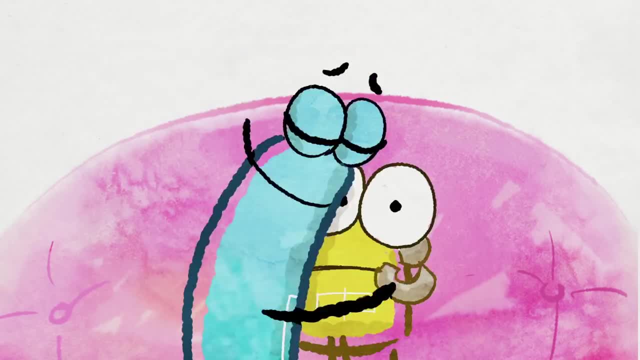 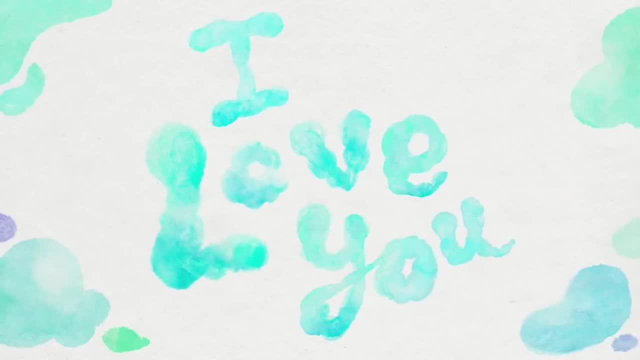 And it really is appealing when you have this loving feeling. So let it out and spread it far and wide, Because love's not just a word but a feeling, have you heard? And you can use it to show how much you care. 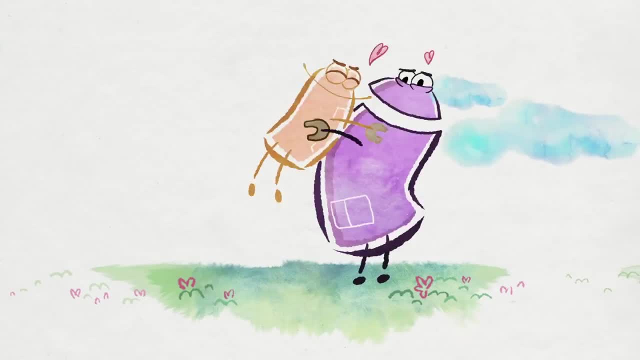 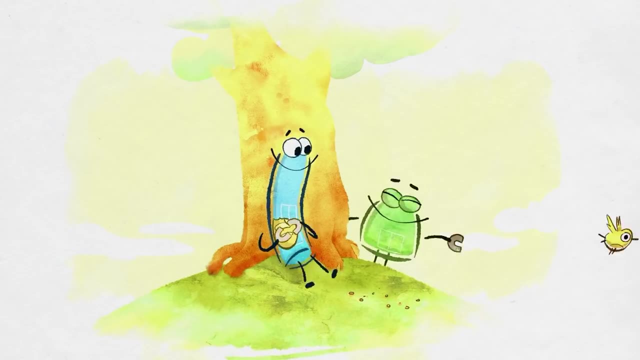 Love. it has no price, but it's extra special and nice. It's the best kind of gift you can share. You love the stuff that brings you joy: your friends, your pets, your favorite toys. You love your family and the thoughtful things they do for you. 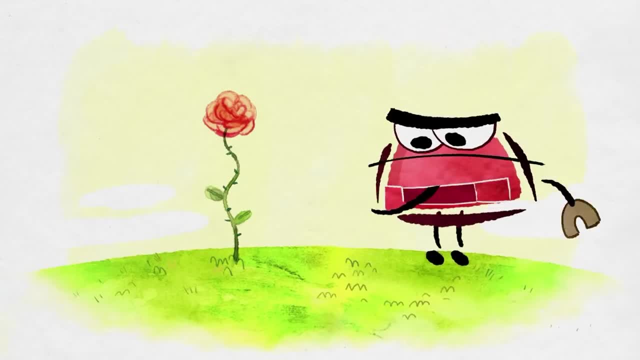 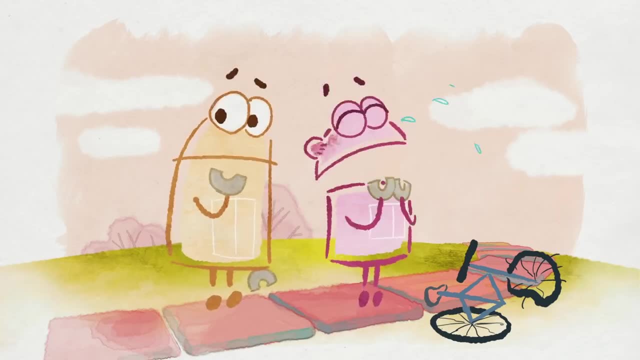 You love to learn to play and sing, You love the time to do your thing, And don't forget to love the one called you, Because love's not just a word but a feeling, have you heard? And you can use it to show how much you care.